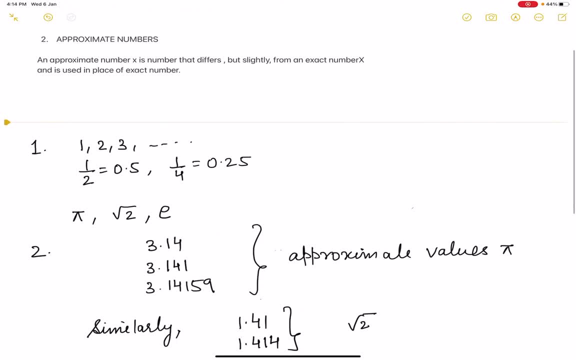 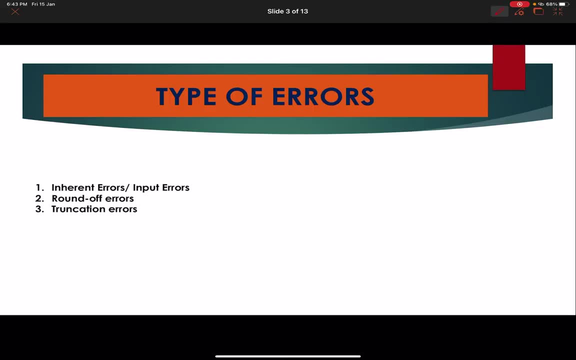 place of exact number, so we may use the approximate number in place of exact numbers. so now let us move to errors, that is, types of error. so the first type of error which we study is inherent error or input error. second is round off error and third is truncation error, so inherent. 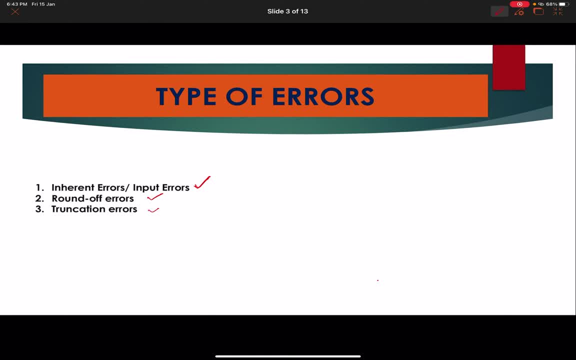 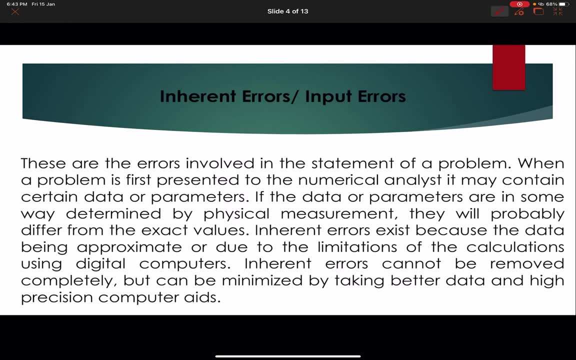 error first is inherent error. so inherent error is already there in the problem statement. so when a problem is first presented to the numerical analyst it may contain certain data or parameter. so this parameter involved can only be determined approximately, so it will give error in the initial, like, for example: 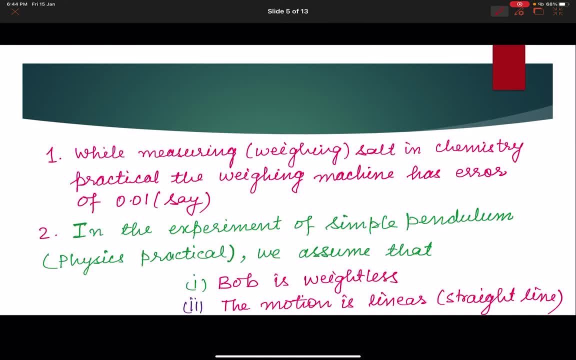 if we consider the are the practical which we did in chemistry of weighing salt, suppose the machine has error of 0.01. so whatever we data collected of 100 or 200 or 10, data itself has an error. so this error, which it is there in the statement of the problem, is called. 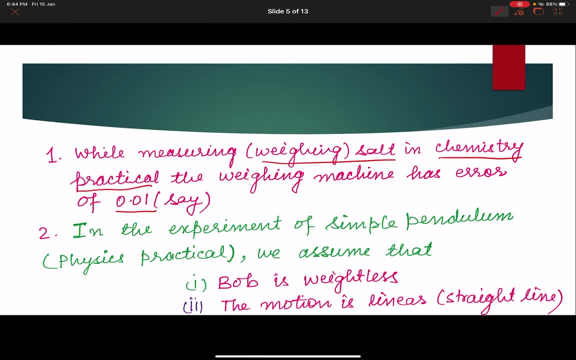 inherent error. let us move to one more example which we, uh the practical, the physics practical, we, in the physics practical, we did this example, we did this uh experiment of simple pendulum and in this we assumed that the bob is waitlist and the motion is straight line. but this is not. 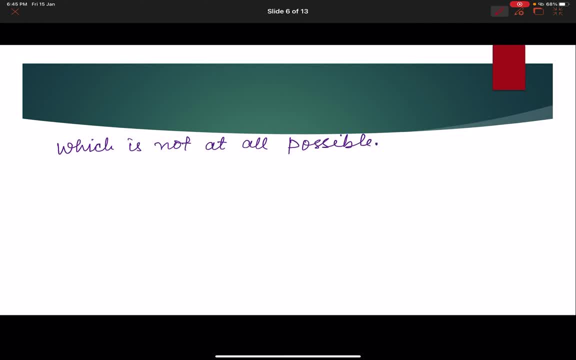 at all possible. so if the motion is not straight line, so the parameters we used cannot be determined and can be only be determined approximately. so parameters can only be determined, determined approximately so, wherever approximation is now there. now, if we move to third problem, suppose i am finding the value of y where we have some value. 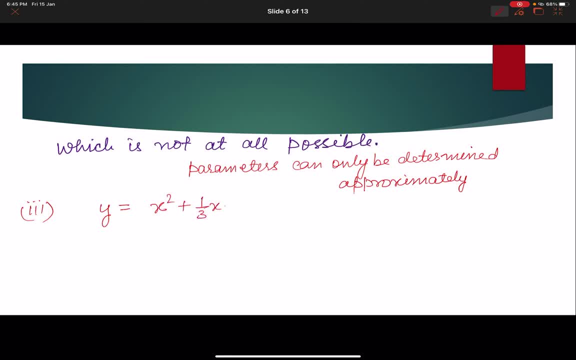 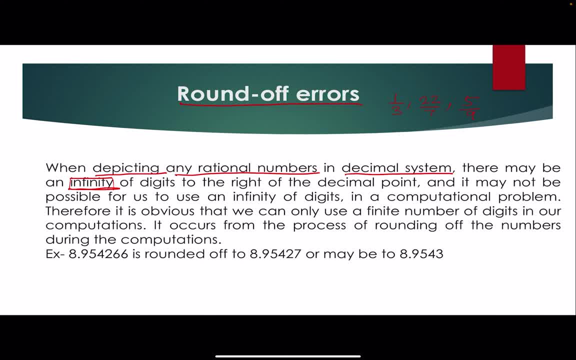 so if i am going to take the value of 0.3 and pi is approximate values, so if i am going creeps in, so it occurs from the process of rounding of the numbers during the computations. for example, in this case, if we take 8.954266- suppose i am using this number in one question- 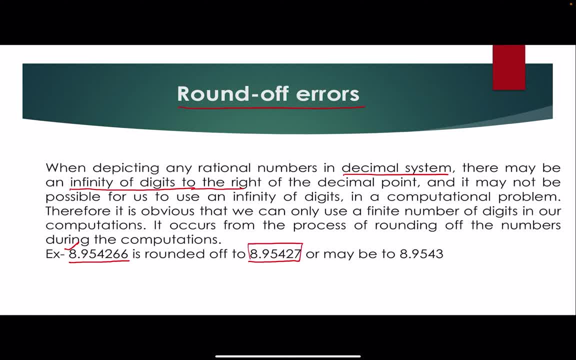 and in another question i am using an approximation of this. so if i am using this one, then the error which will creep in is 8.954266 minus, say, 8.95427, so we can see that there will be an error of this. similarly, if we round off it to 8.9543, then the error involved is is almost: 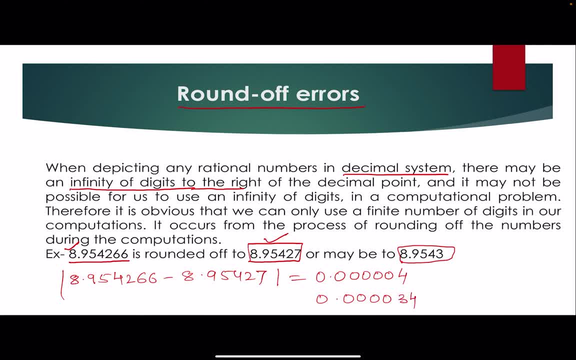 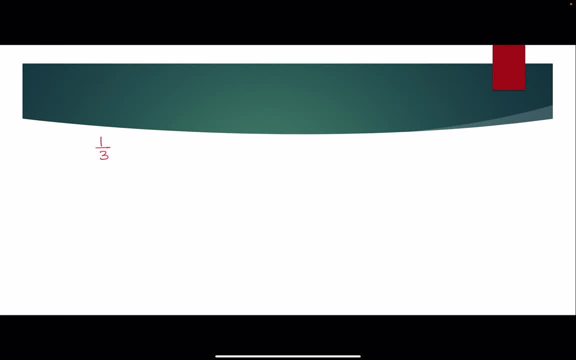 this much. if you remember, in the inherent error section we has used the number one by three, say it has decimal representation in this format. so if we round off this, if say, if we are taking 0.33 as an approximation of one by three, then there will be an error and the error is one by three. 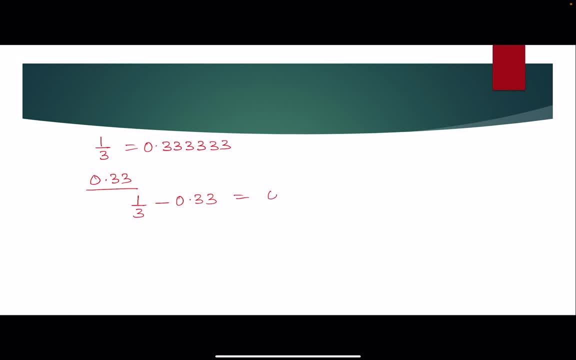 which is equal to zero. so this is the error which will creep in. so if we round off this minus 0.33, and you can see that the error which this time involved is this much. similarly, if i take the approximation as of 1 by 3 as this, then again we have an error and the error is this much. 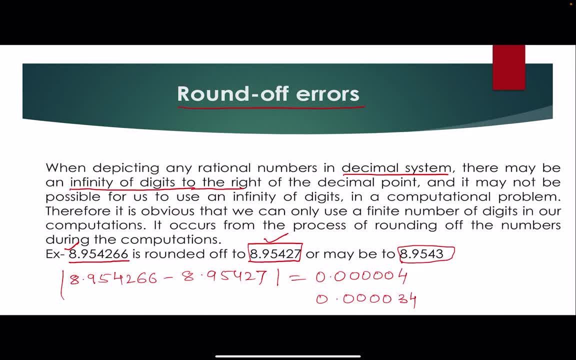 so this round of error basically comes when we are rounding off and approximating the numbers because of our limitation to take the significant number of digits. okay, students, so we may always minimize round of error first. first thing is, while calculation we can take the number, the significant digits, more, and another form is if, say, we may cancel out something. 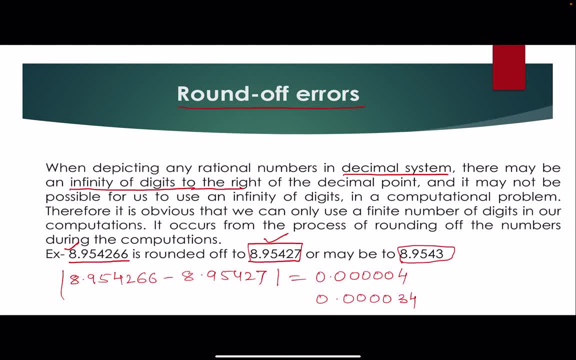 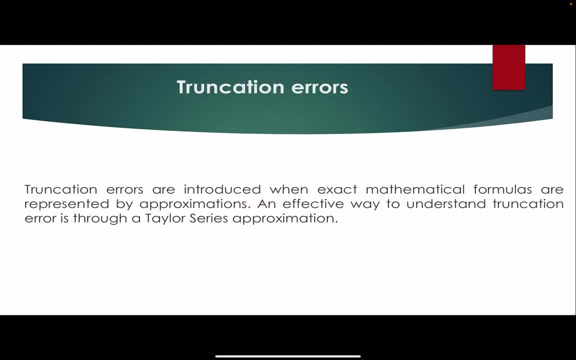 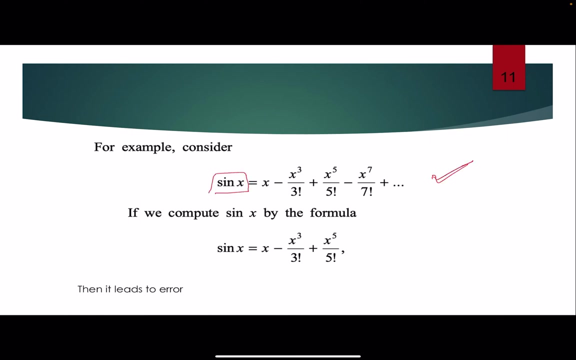 and put the identity, the identity which we are getting, in the correct format, then also round of error may be removed: truncation error. so in numerical method this error creeps in when exact mathematical formulas are represented by approximation. so for example, consider this formula for sine x. so we have this exact formula for sine x. 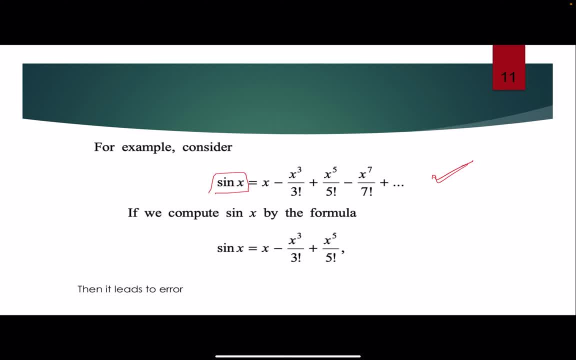 but if we truncate this formula, that is, if we chop off rest of the terms. so if we consider, if we chop off all this term, that is the meaning of truncation. so if it is chopped off, it means that we are taking lesser terms. so we are. 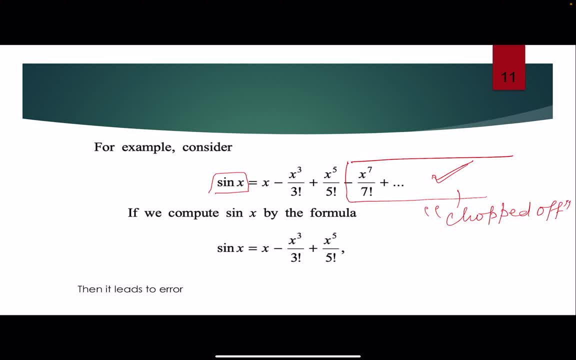 approximating the exact formula and due to this this truncation error comes in. suppose we take the case of e to the power x, so we have the formula of e to the power x as 1 plus x plus, say x, square upon factorial 2 plus x, cube upon factorial 3 plus, so on. so in order to find this, suppose i have to find: 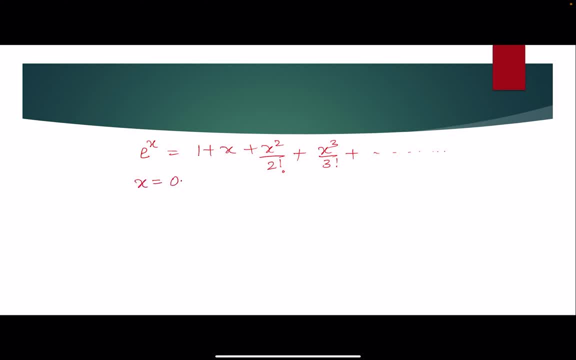 we have to find the value of e to the power x as 0.5, and if we take only the first term- if i take 1 term- then we get the value as 1. if i take first two terms, then i will get the value as. 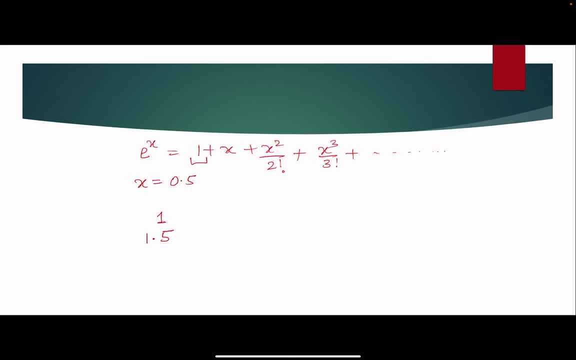 1.5 if we take first three terms. if i am going to take first three terms, then i am going to get the value 1.625. if i will take first four terms terms till here, then i am going to get the value 1.64583333. 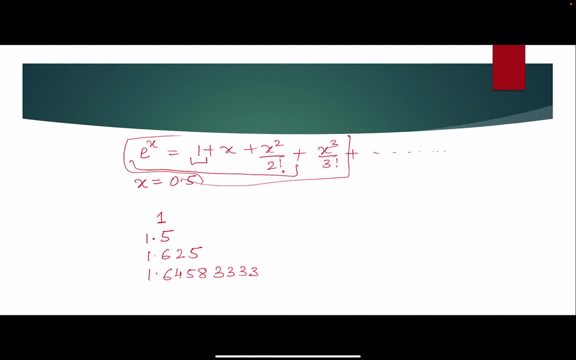 So when we chop off the terms, then the error which comes is called the truncation error. Now, what is the truncated value? Truncation error is the difference between the truncated value and the actual value. A truncated quantity is represented by a numeral with a fixed number of allowed digit. 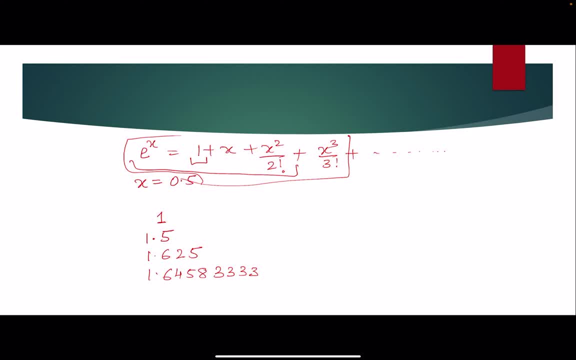 So suppose, if we take another example, if we consider an infinite series, let us consider this series is 1 by 2 plus 1 by 4 plus 1 by 8 plus 1 by 16 plus 1 upon 32.. 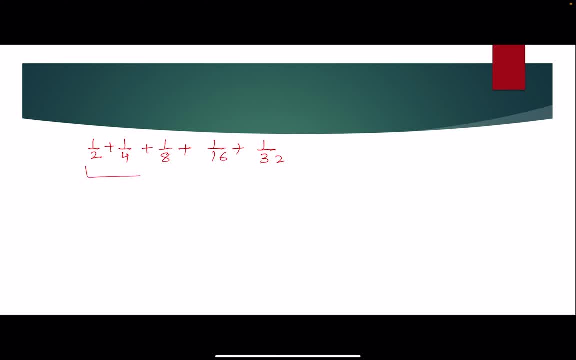 If we chop off the terms, so if we add these, the sum of the series comes out to be exactly 1.. Ok, And however, if we truncate the series, if we chop off the series to only the first four terms, then first four terms are, say, 1 by 2 plus 1 by 4, plus 1 by 8 plus 1 by 16, and this 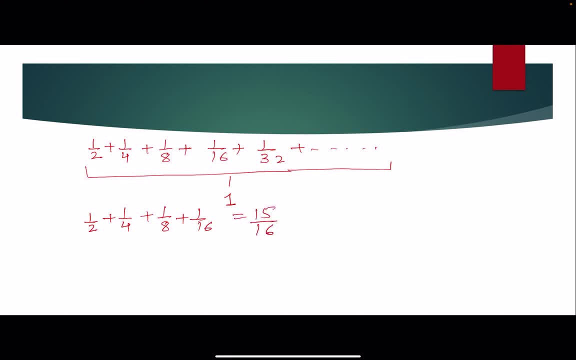 comes out to be 15 upon 16.. And this will create an error, and the error which we get is 1, which was the exact value which we got, And then, taking first few terms, We get 15 upon 16, and so the error which is here is: 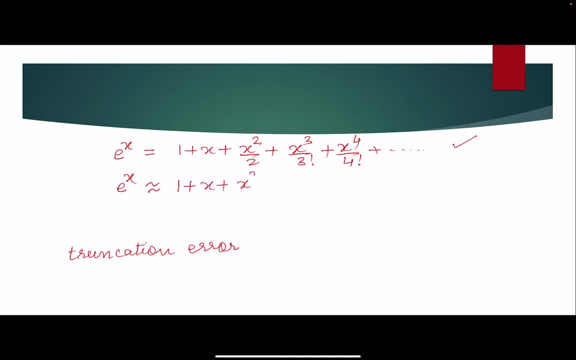 Let us consider e to the power x again. The series expansion of e to the power x is this: and if we take the value of e to the power x is, say, the first three terms 1 plus x plus x square, then what will be the truncation? 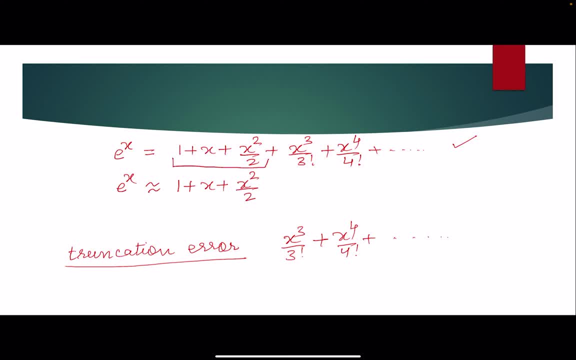 error. in this case it is x cube upon factorial 3 plus x squared. That is our truncation error. We can write the truncation error as we have taken the truncation error from the expression of the value x to the power of x. 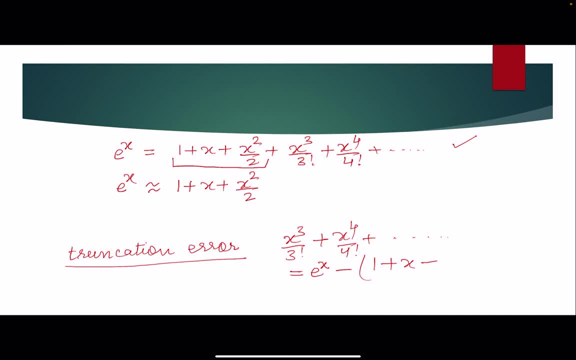 x4 upon factorial 4 plus so on. so if we take these terms only, then the truncation error which we wrote here is e to the power, x minus the first three terms. this is factorial 2. now moving to the definition of error. we have three definitions of error in three ways. we 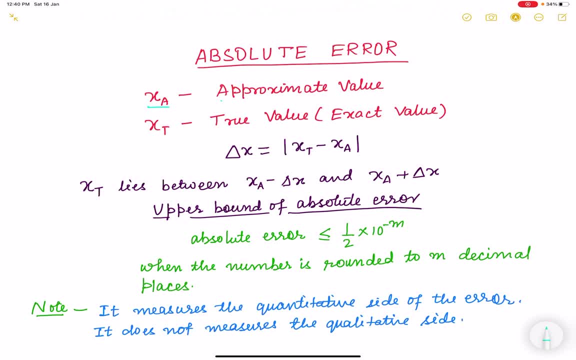 measure error. first is absolute error, second is relative error and third one is percentage error. let us discuss all three in details. absolute error: so if we assume x a as the approximate value and x, t, t denotes for the true value or we call it an exact value, then the absolute error we 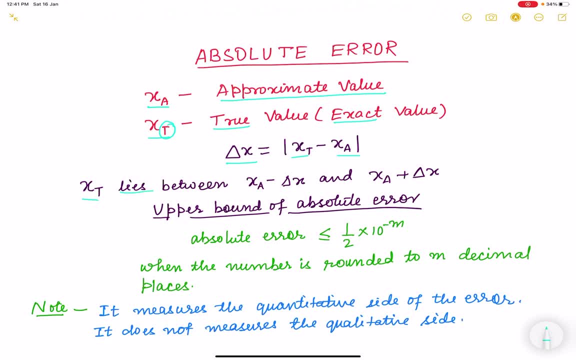 denote it by delta: x is x, t exact value minus the approximate value, and this is the absolute value of the you difference. so we can say that the true value, or the exact value, lies between approximate minus this absolute error, and approximate plus absolute error. what is the upper bound of this absolute? 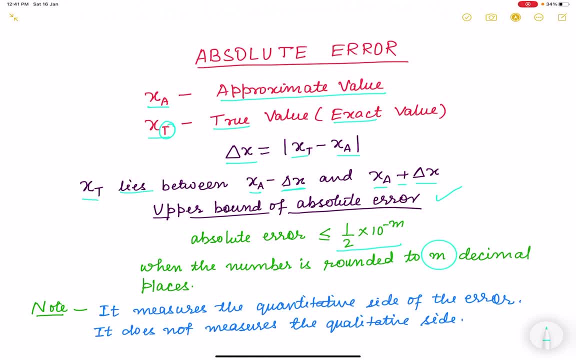 error. it is 0.5 into 10 power minus m, where the number is rounded or rounded off to m decimal places. so the number, if the number is rounded off to m decimal places, then the absolute error is 0.5 into 10 power minus m. what is the main thing about this absolute error? is it measures quantitative? 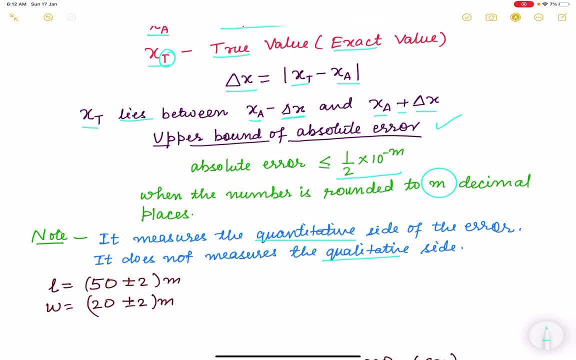 side of the error. as far as qualitative side is concerned, it doesn't measures the qualitative side of the error. to understand that the absolute error measures more quantitative side of the error than the qualitative side, let us consider a cross section where the length is 50 and the width is 20. 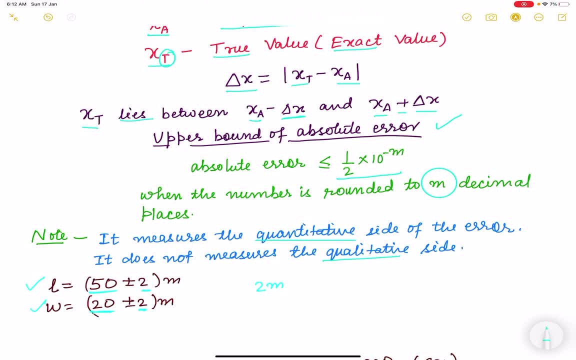 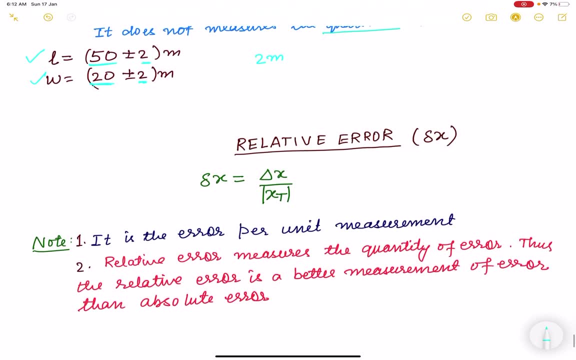 where the error involved is 2. so if you measure the absolute error in both the cases, the absolute error will come out to be 2 meters, but the actual error is more than this. if you measure it for the whole cross section, it is more than this. so we move to the relative error. it is denoted by delta x, and delta x is equal to. 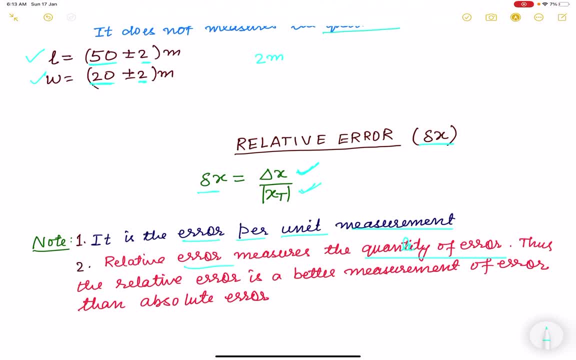 absolute error. divided by the true value, it is the error per unit measurement. here we take unit measurement and relative error measures the quantity of quality of error. it measures the quality of error and we may say that relative error is a better measurement of the error than the absolute error. relative error is more better. 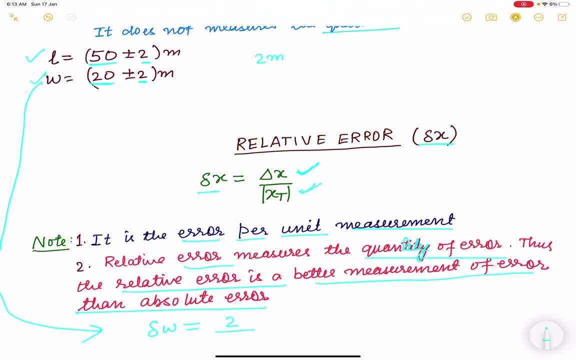 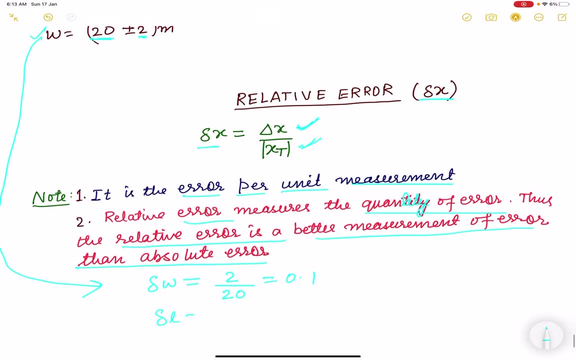 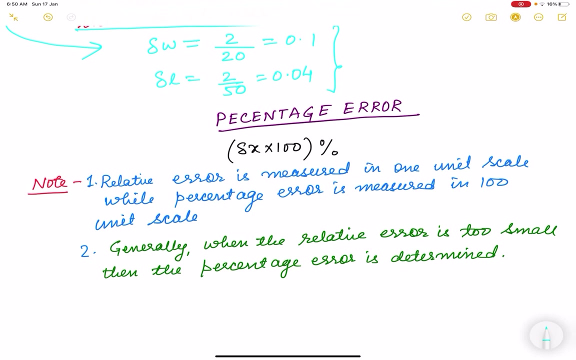 than the absolute one. if we consider the same example which we considered here, in this case the relative error is given by: as for width, it is, since the absolute error is 2, so it is 2 upon 20, which will come out to be 0.1. similarly, for length, it is 2 upon 50.. in both the cases, you will find. 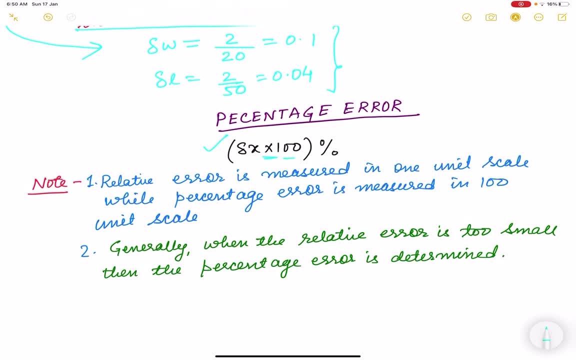 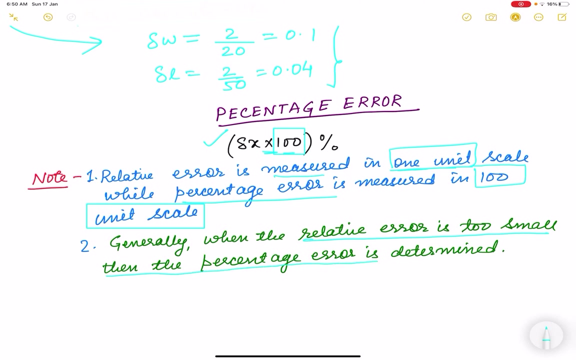 that the relative error is much better. Moving on to the percentage error, error multiplied by 100. so that is how we find the percentage relative error is measured in one unit scale and if we consider percentage error, then it is measured in 100 unit scale. so this is the difference between relative error and the percentage error. 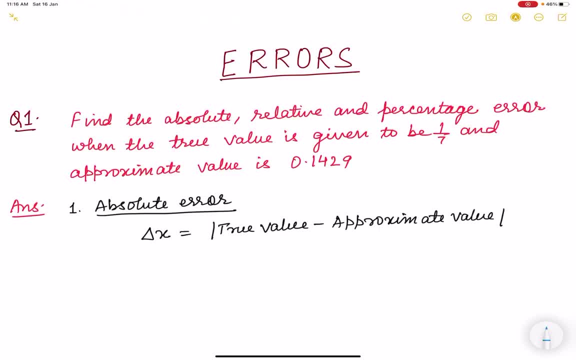 so, generally, when the relative error is too small, then we find the percentage error. and now let us move to the questions we have. first question on errors. we have to find the absolute, relative and percentage error when the true value is given to be 1 by 7. 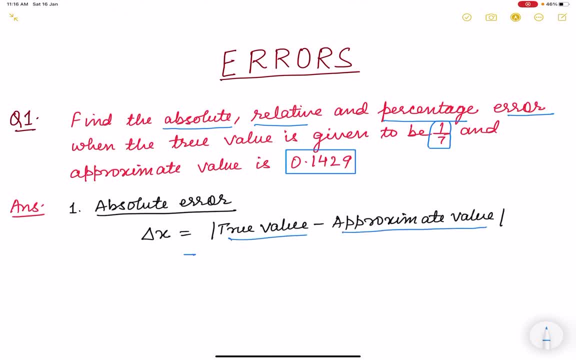 and the approximate value is 0.129- 0.1429. so formula for approximate absolute error is true value minus approximate value. so the true value is given to be 1 by 7 and the approximate value is 0.1429 and on calculation this will come out to be around 0.000043.. 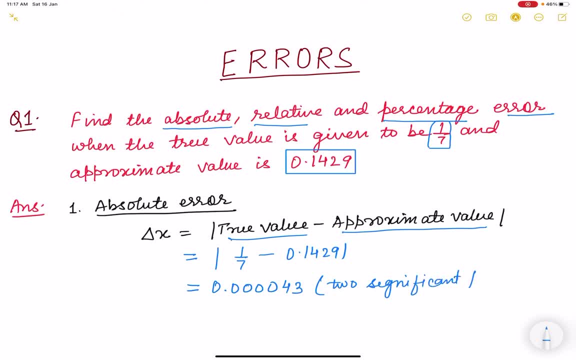 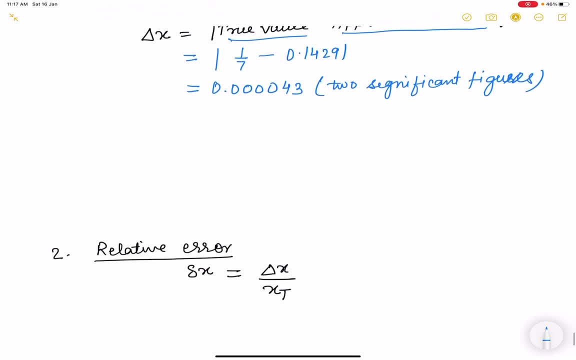 and this is rounding up to two significant figures. this will rounded to two significant figures. moving to relative error, relative error is absolute error divided by the true value. so if we take the absolute error, as we found earlier, it is zero point 0, 0, 0, 0, 4, 3, and divided by the true value, which is 1 by 7, and this will come out. 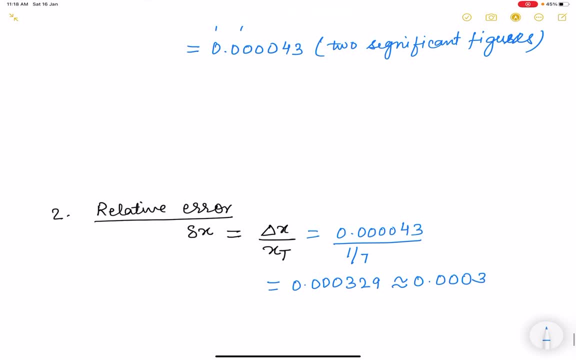 to be 329, mimicking the approximate value as 0, point. ok. now moving to relative error: relative error, which is absolute error divided by 0, or to percentage error, and percentage error is relative error, which is that is, we are finding the percentage, so relative error multiplied by 100. so if we take this relative error from 0.2.